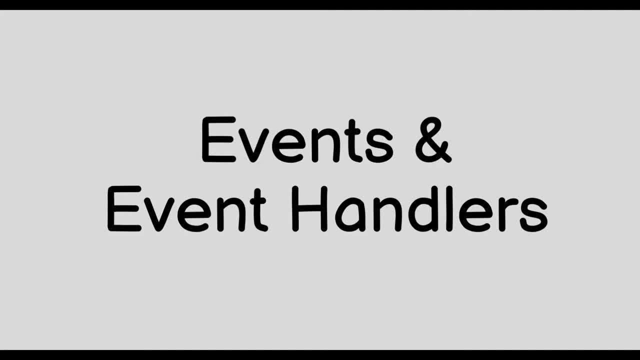 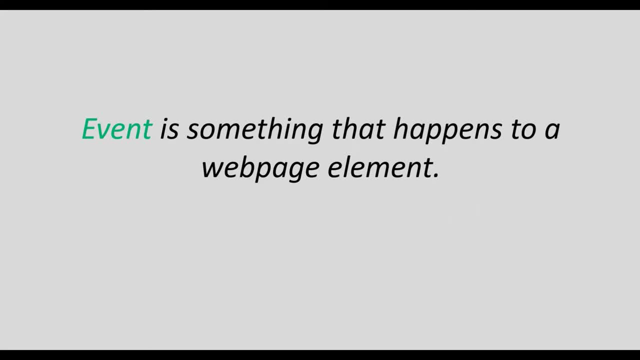 JavaScript is an event-driven programming language. That means in JavaScript we mostly write programs which will respond to an event. In JavaScript, events are something which happens to a web page element. For example, when a button is clicked, the click event happens. 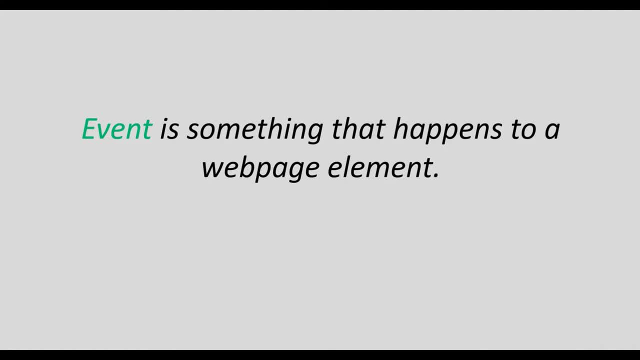 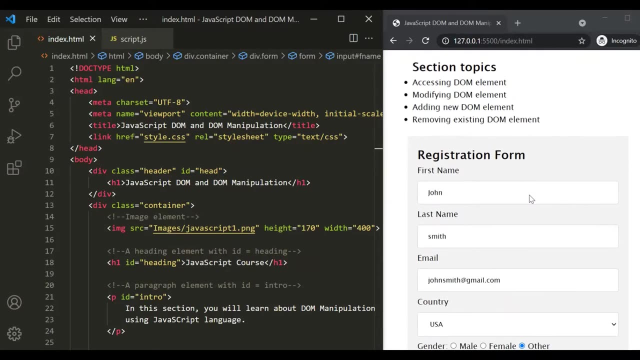 Similarly, when a text box is focused, a focus event happens, and when a key is pressed on the keyboard, a keypress event happens. We can write JavaScript programs to react to these events and this is called as event handling. So in this web page, when I click inside this text box, 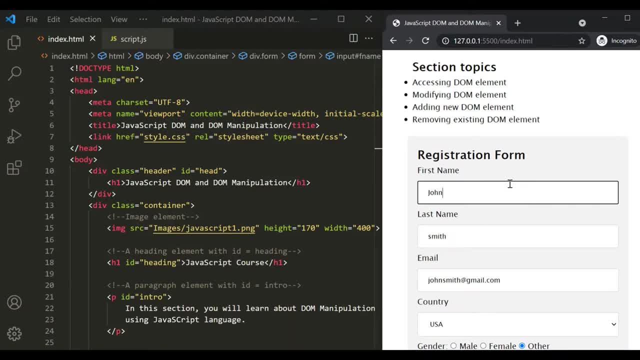 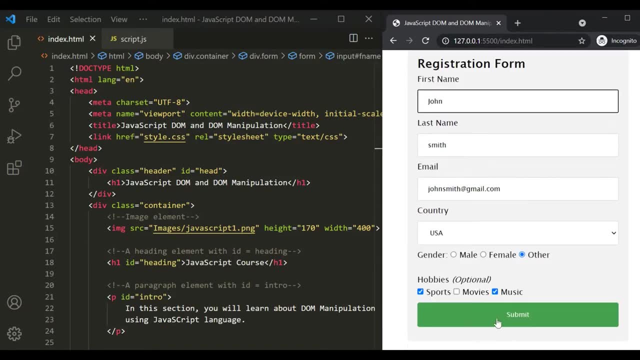 a focus event will happen on this text box. Similarly, when I hover over this H2 element, in that case mouse over event will happen. and when I click on this submit button, a click event will happen. We can handle these events by executing a piece of JavaScript code. 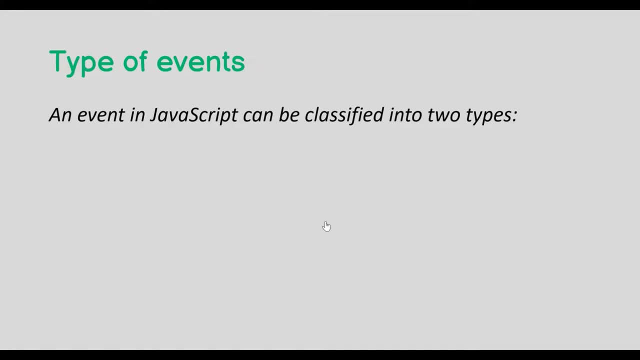 and then showing some response to the user. In JavaScript, an event can be classified into two types: Browser-specific events and Dome-specific events. Browser-specific events happens on the browser. For example, resizing browser window, scrolling up and down, etc. are browser-specific events. 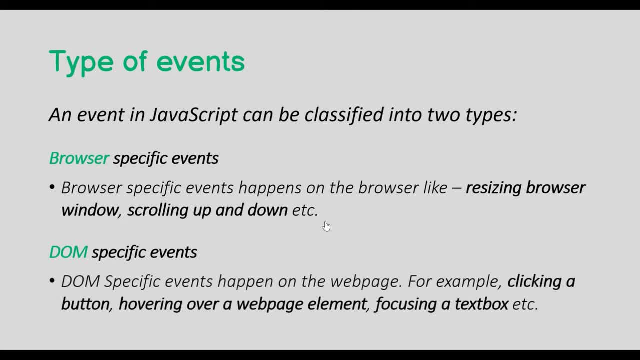 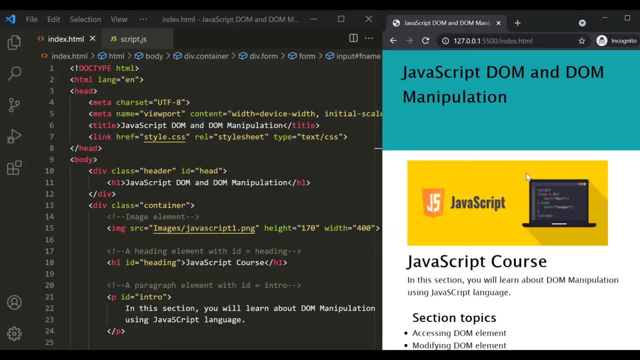 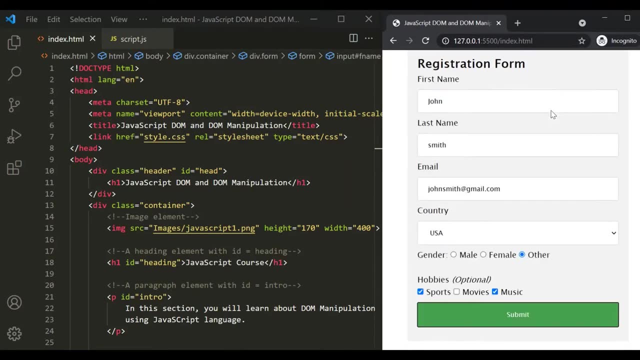 On the other hand, Dome-specific events happens on the web page, For example, clicking a button hovering over a web page element focusing a text box, etc. So here, when I resize this browser window, it is a browser-specific event. Similarly, when I scroll down or scroll up, 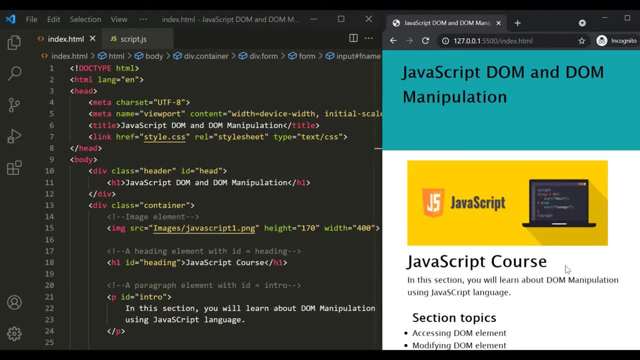 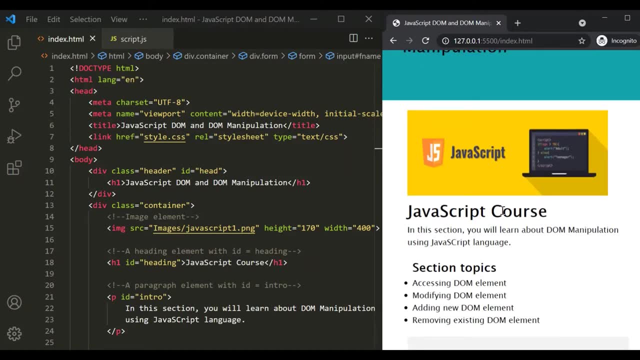 it is also a browser-specific event. On the other hand, when we do something on a web page element, that is Dome-specific event. For example, when I put my mouse over this H1 element, this is a Dome-specific event. Similarly, when I click inside this: 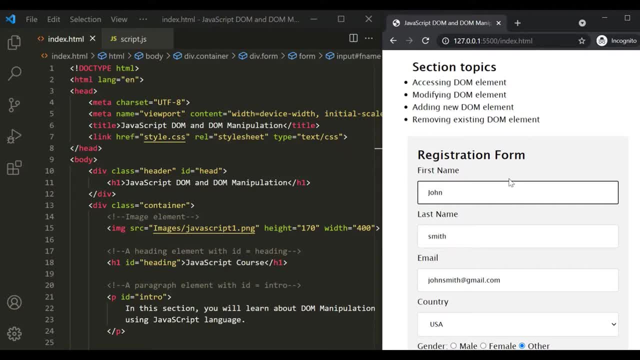 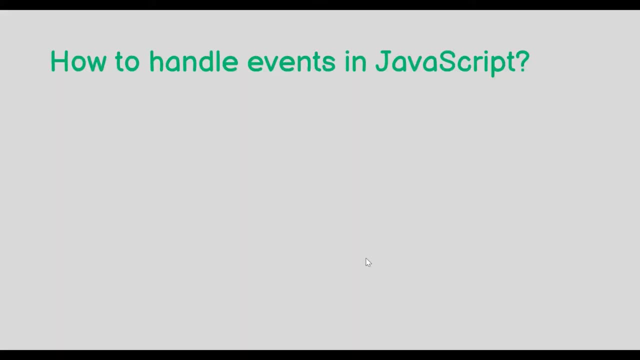 text box. it is again a Dome-specific event because here we are doing something on a web page element. We can write JavaScript programs to listen to these events and when that event happens we can show some response to the user. There are several ways to handle events in JavaScript. For example, we can use inline. 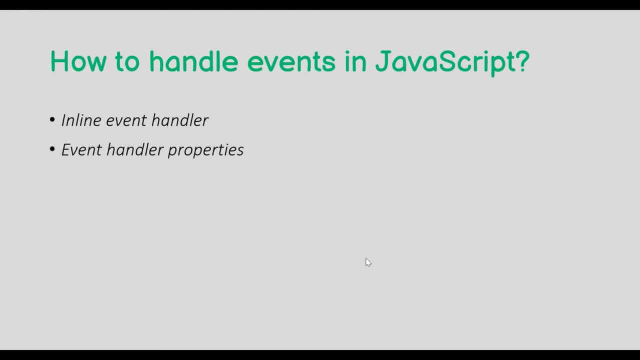 event handlers. we can use event handler properties or we can also use addEventListener method to listen to these events and then, when this event happens, we can show some response to the user. Now in this lecture we will mainly focus on inline event handlers. 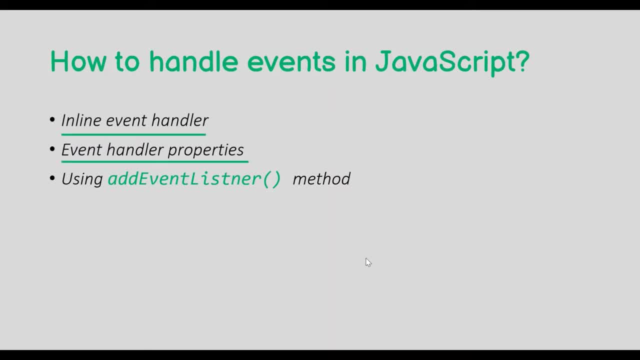 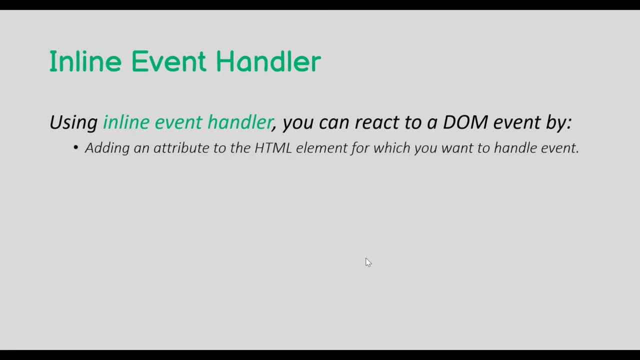 and event handler properties. Using inline event handlers, you can react to a Dome event by adding an attribute to the HTML element for which you want to handle the event. The attribute name must be the event name prefixed with on. For example, if you want to handle focus event, then the attribute name should be onFocus. 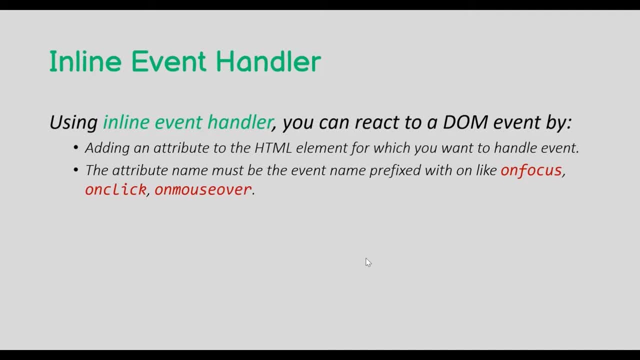 If you want to handle click event, then the attribute name should be onClick, And if you want to handle mouseover event, then the attribute name should be onMouseover. Then we can assign any JavaScript expression to these attributes which will be executed when that event happens. Let's understand this with an example. 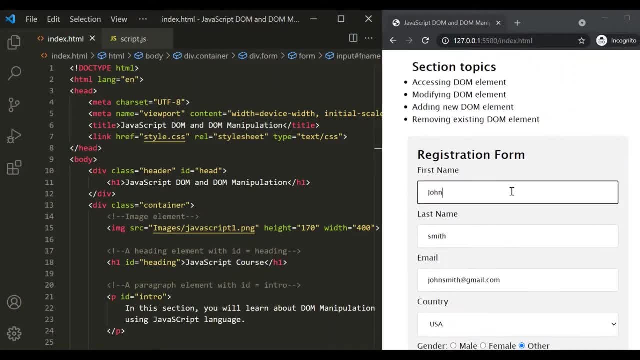 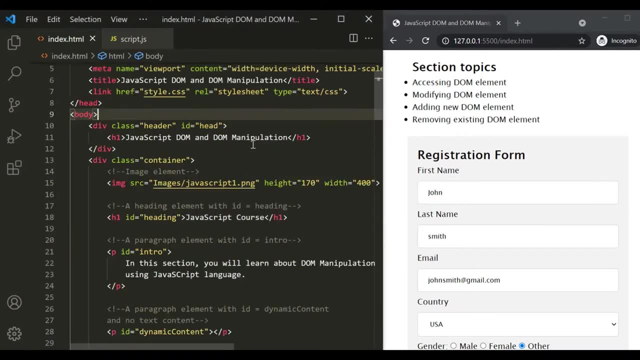 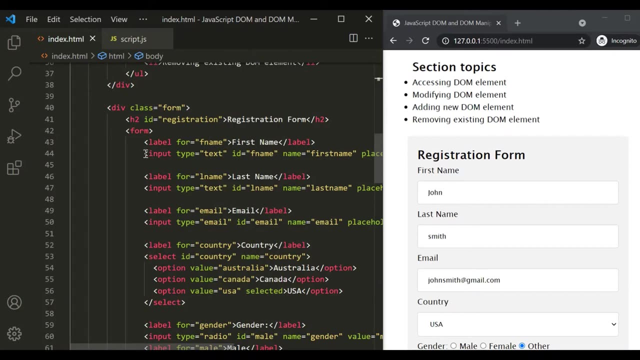 Now in this web page, let's say we want to handle this focus event on this first name text box. So in the indexhtml let's first find the HTML element which is displaying This text box. So if we scroll down here, we have this form and inside this form we have this input. 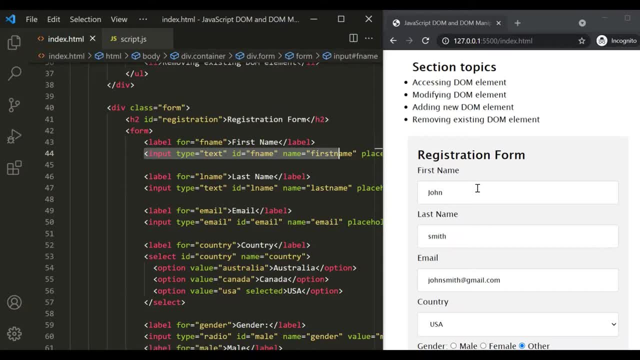 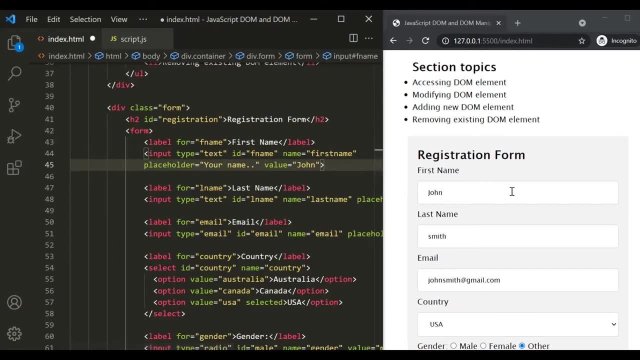 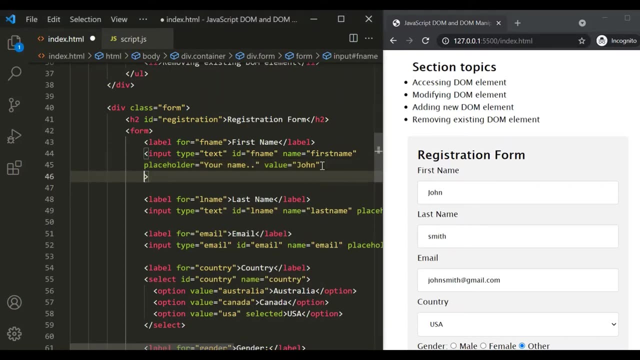 element, And it is this input element which is displaying this text box in the web page, So let me move it to the separate line so that it will be more readable. Okay, Now, if we want to handle a focus event for this text box, then we can add an attribute to this input element And 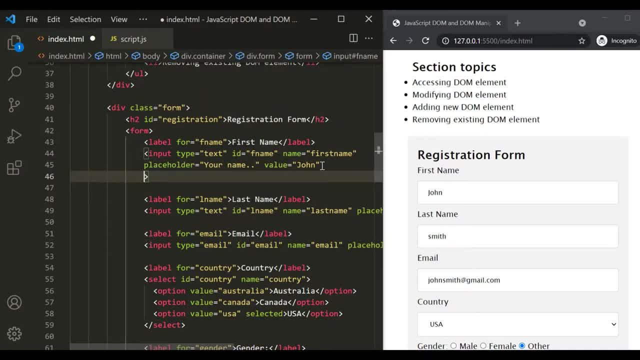 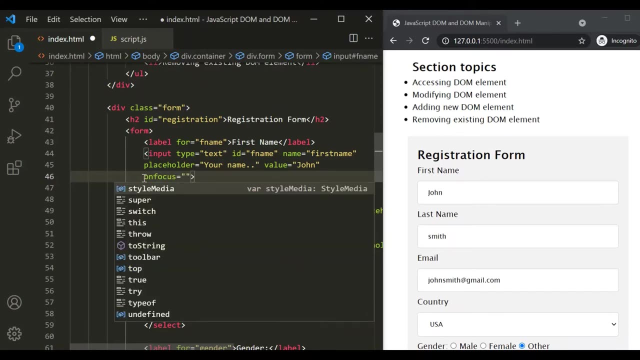 the name of the attribute should be the event name which we want to handle, prefixed with on. So here, let's say we want to handle focus event, So the attribute name should be onFocus. Okay, Now to this we can assign any JavaScript expression which will get executed when that event happens. 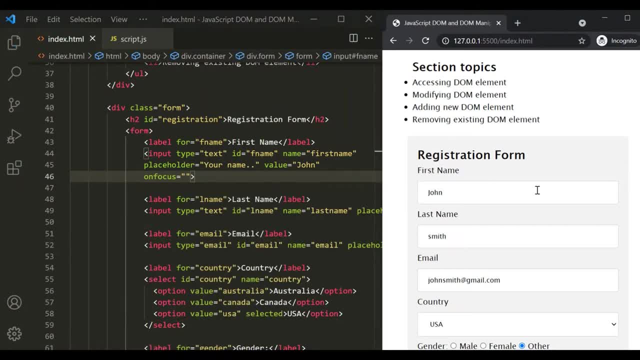 So let's say, when the focus event happens for this text box, we want to change its background color to yellow. Okay, So we can write a JavaScript code inside these codes in order to change the background color. So we can say: 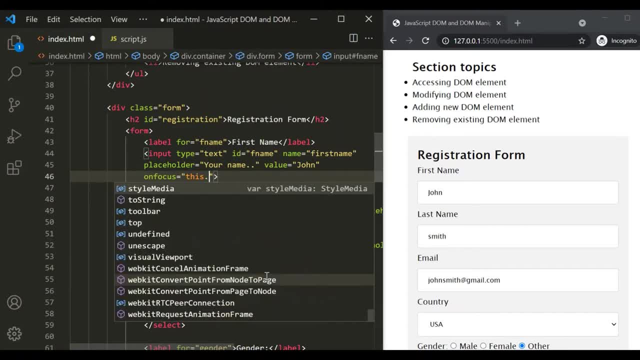 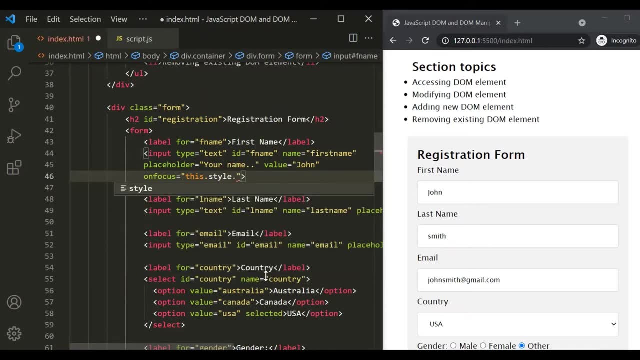 this dot, and here we want to change the style. So on this property, I mean on this object, let's call style property, And to that let's set the background color, And let's set the background color to yellow. 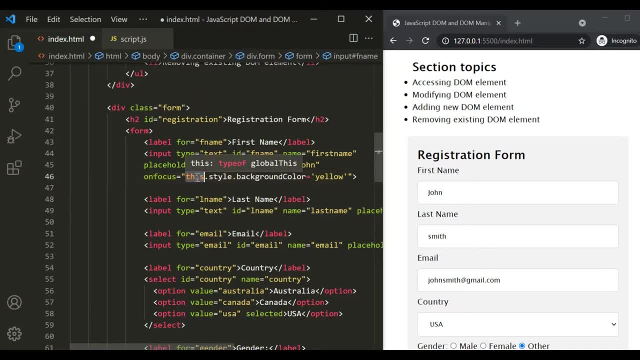 Now here, this variable will point to the- to this first name text box object. Okay, So in the dome an object will be created for this text box, And when we are using this keyword on the input element, this here refers to the. 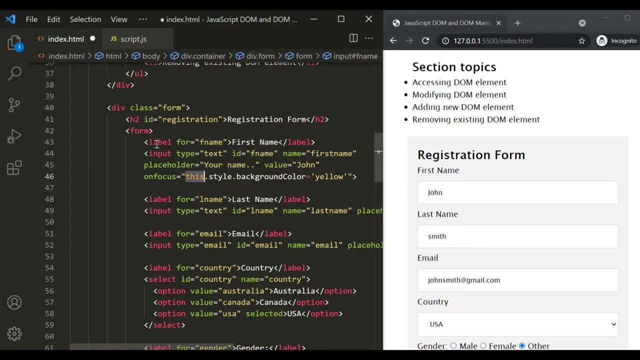 dome object which represents this text box, this input element in the dome. Okay, So here on that object we are calling the style property and then we are setting the background color to yellow. Let's save these changes, Let's click inside this text box. So here a focus event will happen. And when the focus 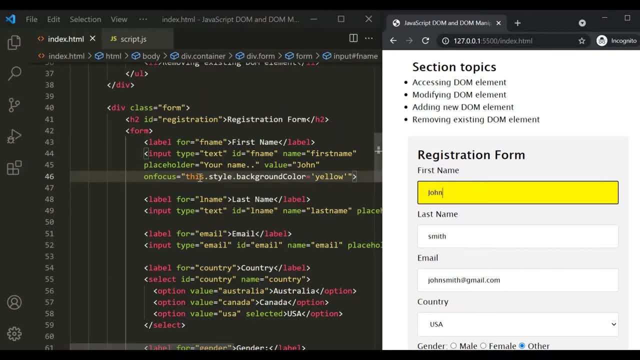 event happens. we are assigning a JavaScript expression to this on focus attribute, So this expression gets executed when this focus event happens, And that's why the background color of this text box has changed to yellow, And in this way we can add as many events as 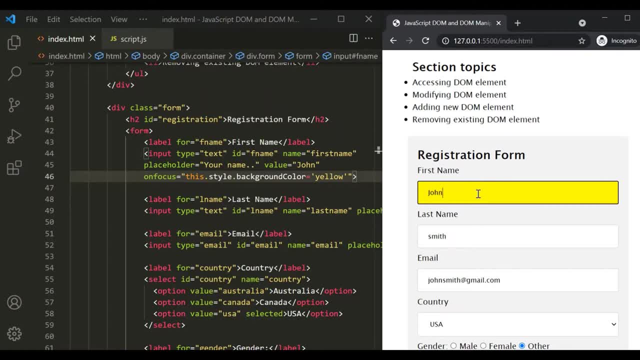 we want to a given dome element. So here we have added only one event to this, only one event Handler, which is focus. Now let's say, when this text box loses its focus- that means when I click somewhere else in the web page- in that case it will lose its focus. So in such case, 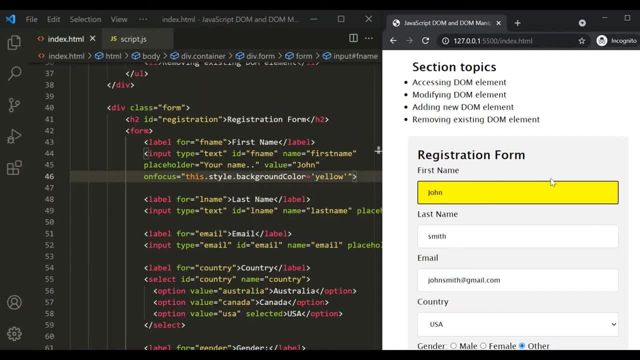 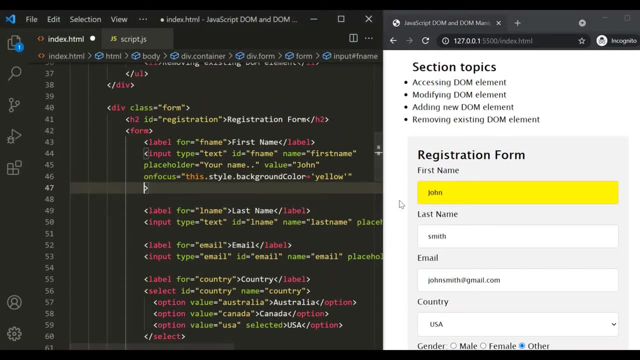 a blur event happens. And when the blur event happens, we want to change its background color back to white. Okay. So again, here let's also handle blur event. So let's say on blur: Okay, And to this let's again assign a JavaScript expression. So again, let's say this: 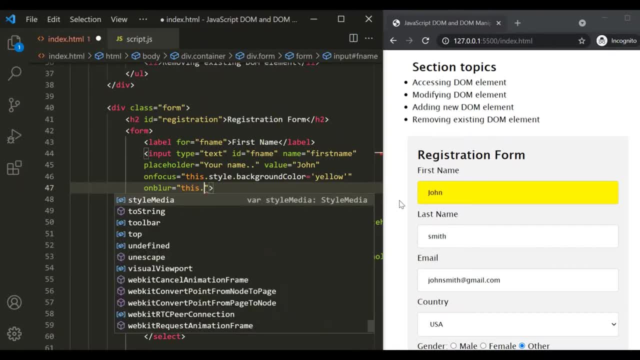 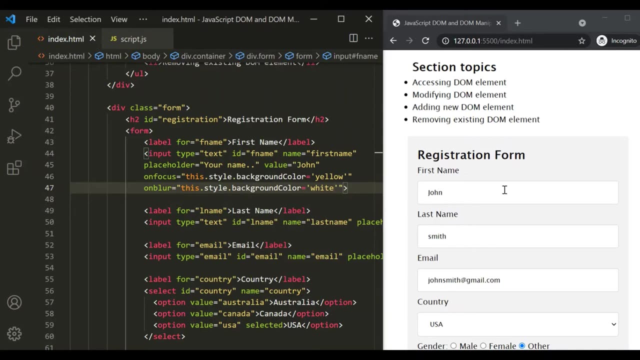 So this here will point to this first name text box And again we want to change the style And we want to set the background color and we want to set it to white, So white. Let's save the changes. Now, when I click inside this text box, focus event will happen And this: 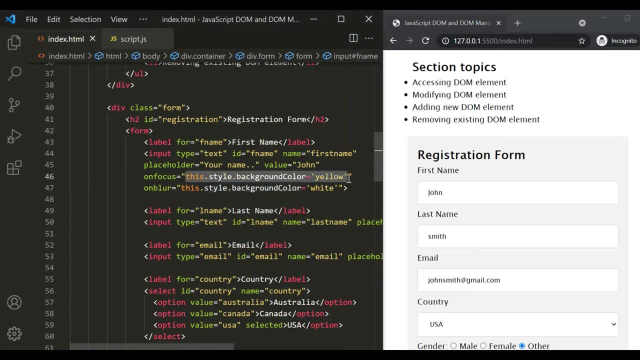 JavaScript expression will get executed and it will change the background color to yellow. and when this text box loses its focus, in that case blur event will happen and blur when blur event happens, this javascript expression will be executed. so if i click somewhere else on the 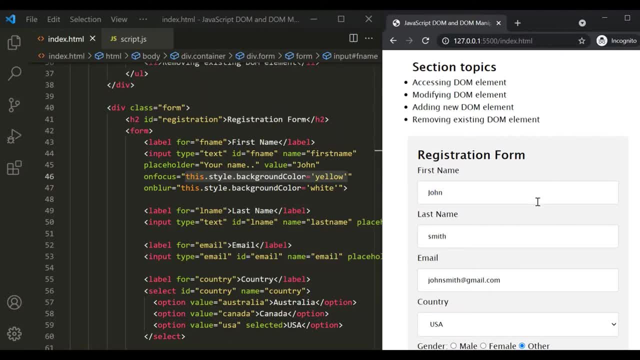 web page. here you can see blur event happens. this text box loses its focus and its background color is now changed back to white. okay, so here for this text box, we are handling two events: focus event and blur event- and we are doing that by using inline event handlers, by adding event. 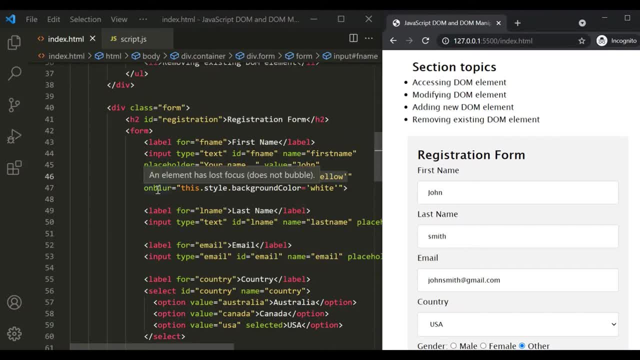 attributes to this input element. now, although the inline event handlers clearly works, as we have just seen, they should not be used in in your javascript program. and why is that? that is because it makes our code messy by mixing html and javascript together. so here in this indexhtml, 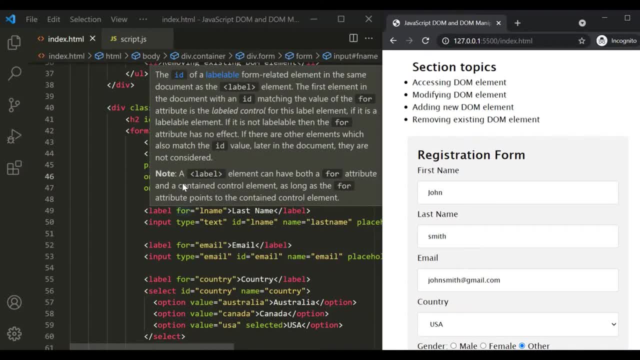 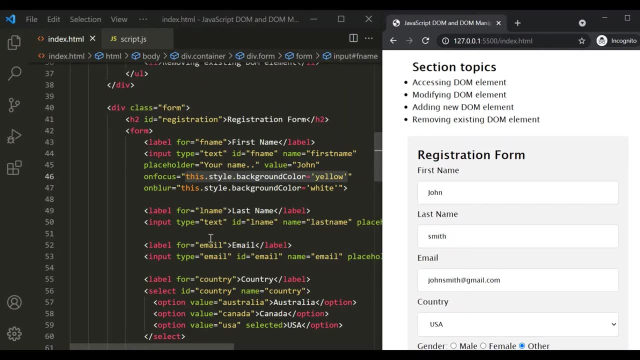 we have html codes and in the html code we are also mixing javascript codes like this: okay, so in this way we are making this html code less maintainable, and it is always a good practice to separate your html code from your javascript code. in that way, the code will be much more. 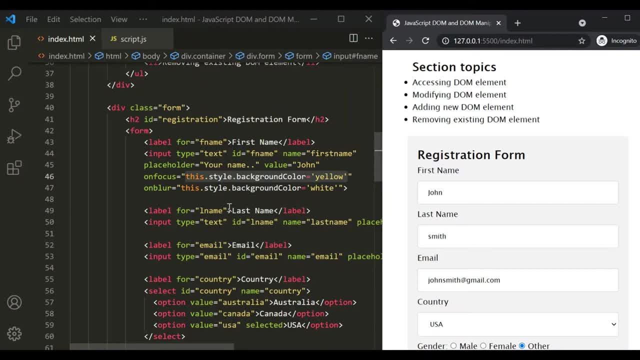 maintainable. now, how can we do that? well, you have. we have learned that when an object is created for an html element in the dome, all its attributes are created as its property right. so here, for this input element, an object will be created in the dome and on that object 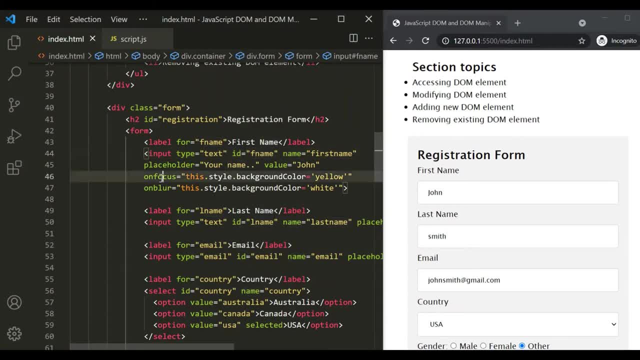 this type, this id, this name, this on focus and on blur, these will be created as its properties. so what we can do is, instead of assigning an attribute to these html elements, we can directly attach a property to the dome object itself. okay, and then we can handle events. let's see how to do that. we can do that by using event. 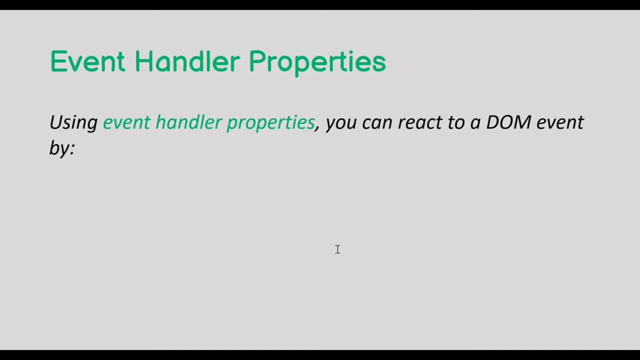 handler properties. so using event handler properties, you can react to a dome event by adding a property to the dome element for which you want to handle event, and then the property name must be the event name, prefixed with on, for example on focus, on. click on mouse over. 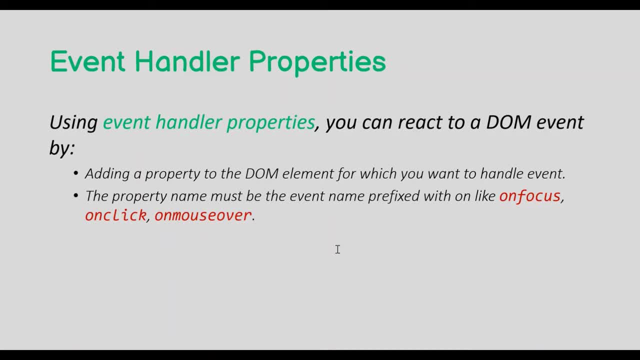 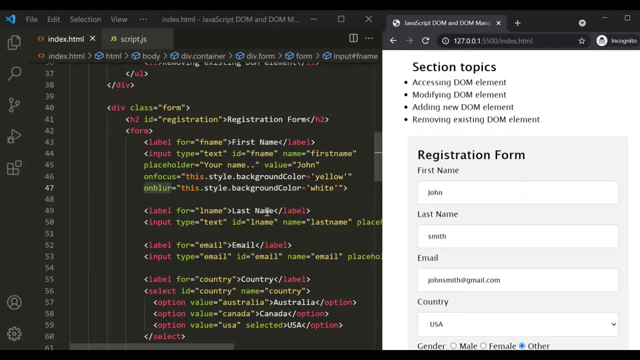 just like we have done with inline event handler, and then we can assign a javascript function to that property which will get executed when that event happens on that element. let's understand this with an example. so here we are handling the focus event and blur event on this first name text box. now let's handle 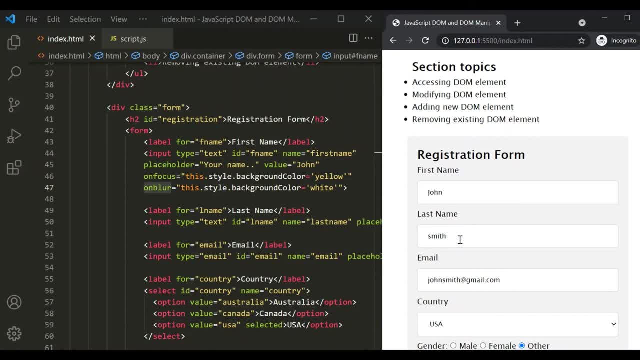 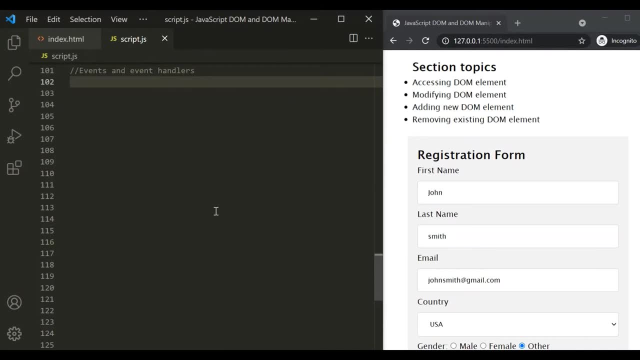 the focus and blur event on this last name text box, and this time let's use event handler properties to do that. so let's go to scriptjs file, and here we are going to handle the focus event and blur event. and here the first thing which we need to: 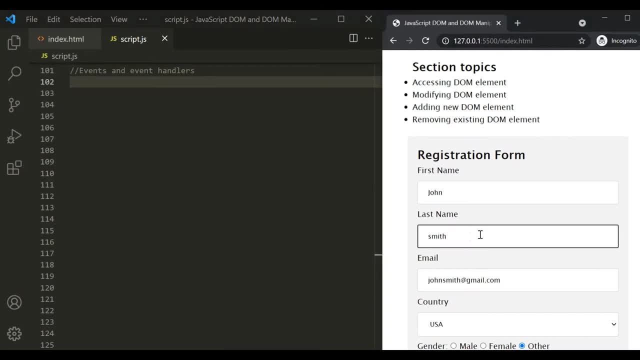 do is we need to get access to this last name text box. okay, so this last name text box will be created as a dome object in the dome so we can use getElement by id method or query selector method to get access to that object. so let's say, documentgetElement by id and. 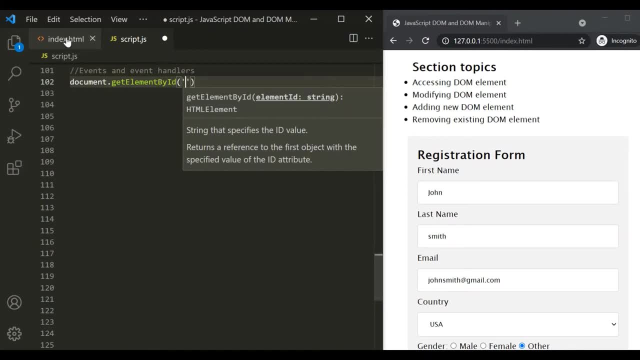 to this: let's pass the id of this last name text box. so let's go to indexhtml and id: this text box is l name, so let's copy this and let's pass it to scriptjs file. okay, so in this way we will get access to this last name text box. let's store it in a variable. 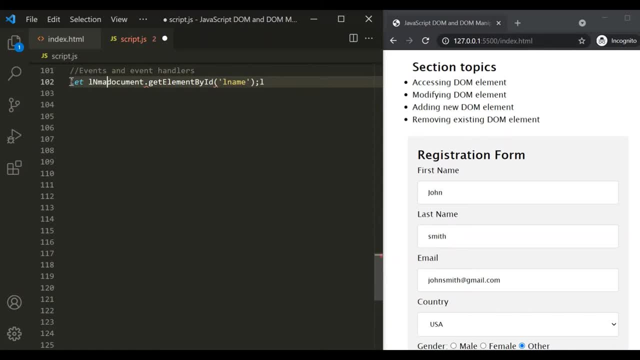 and let's call it l name. okay, now we want to handle focus event for this last name text box. so on this l name, let's attach a property called as on focus. okay, and to this now we can assign a javascript function, and this function will get executed when the focus event is allotted to the last name text box. 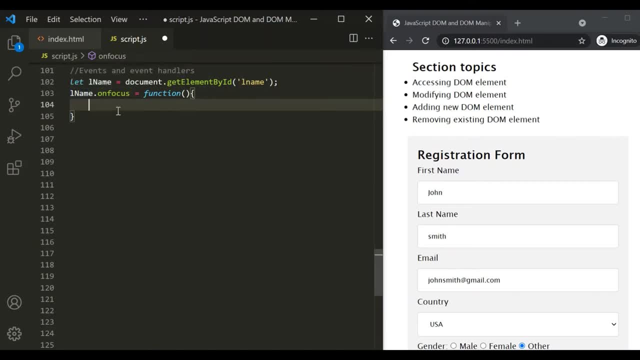 and the focus will get executed when the focus event is allotted to the last name text box. event happens on this last name text box. now what do we want to do here? we want to simply change the background color of this last name text box to yellow when the focus event happens. so let's say: 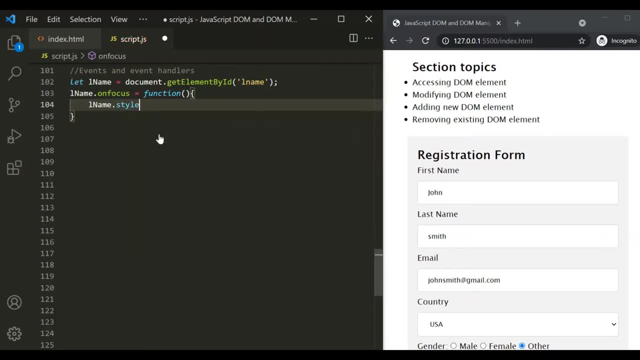 lname dot style, dot background color, and let's set it to yellow. with this, let's save the changes and when i click inside this text box, you can see its background color has changed to yellow. so here we are handling the focus event using event handler properties. okay, and for first name text box, we are: 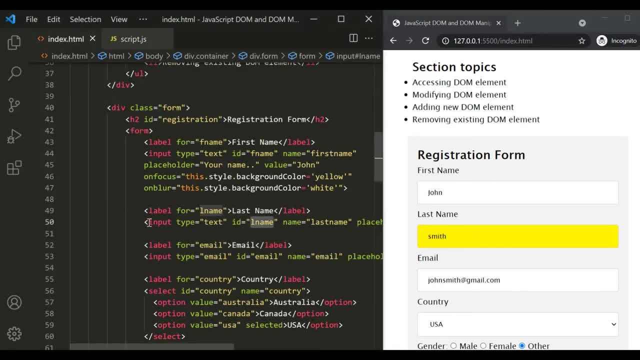 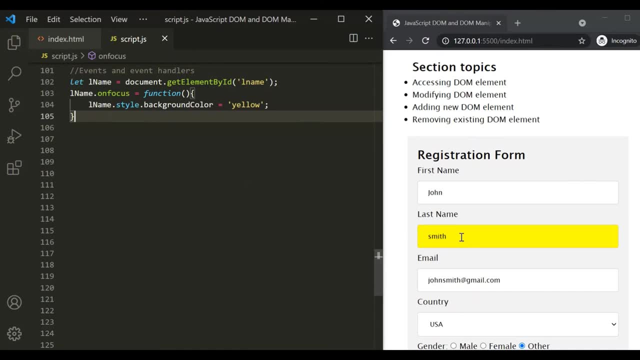 handling this focus event using inline event handlers. that means event handler attributes. okay, let's also handle the blur event on this last name text box. so for that again on the lname we will have to attach a new property and the name of the property should be on. 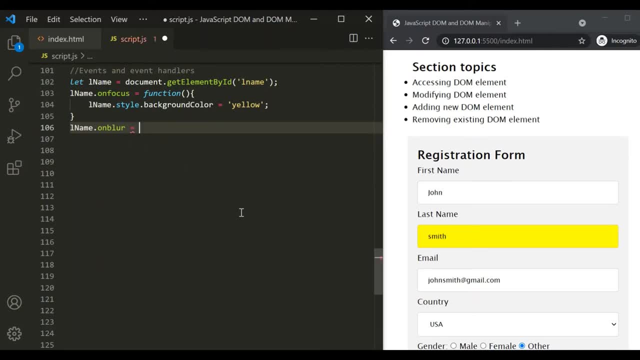 blur, so the event name prefixed with on, and to this again we can assign another function, and here we want to change the background color of last name to white when the blur event happens. let's copy this line of code from here, let's paste it here and let's change the background color to. 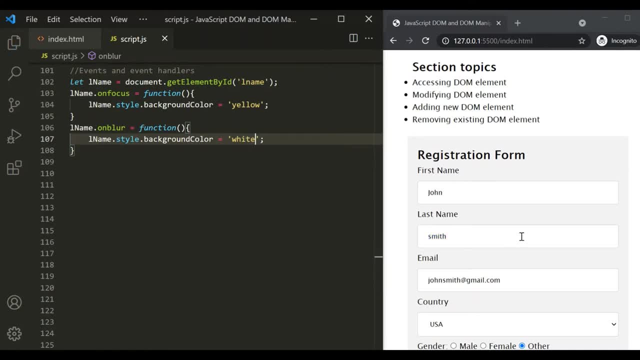 white. let's save the changes. now, when we when the focus event happens on this last name, its background color changed to yellow, and when the blur event happens, its background color now changed to white. okay, so here we are handling the focus event and the blur event using event handler properties, and in this way we are also separating the javascript. 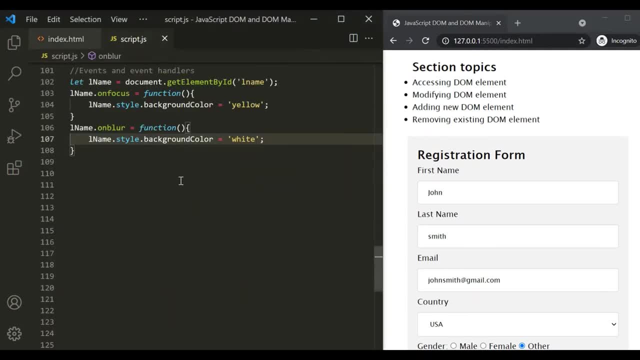 code from html code. okay, so in this way we are making the code more maintainable and also the code is more cleaner. we have separated html from javascript. now, before i wrap up this lecture, let's take another example. so let's say, when we hover over this h2 element, we want to change its color to red, and when we 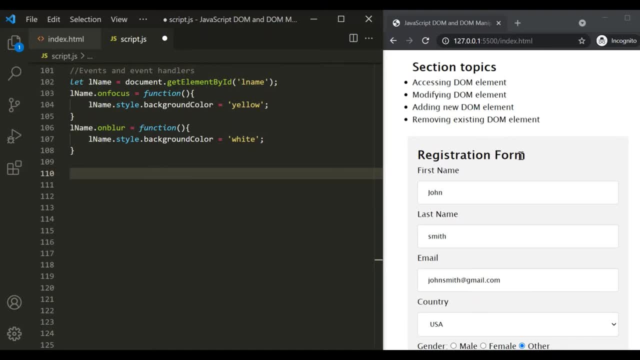 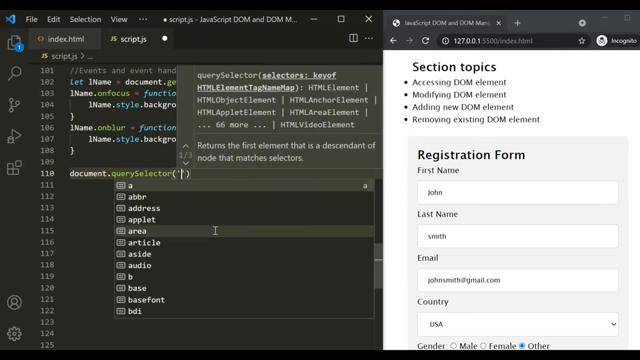 move our mouse away from this h2 element, then its color should change back to black. okay, so we can say: first we need to get access to this h2 element, so for that let's use query selector method. so query selector, now you can use document get element by id method as well, but here i just want to use this query selector method. 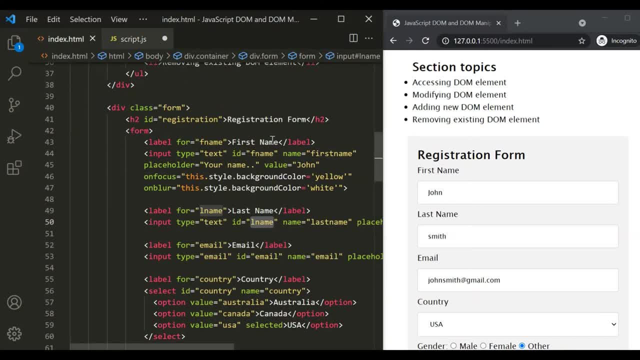 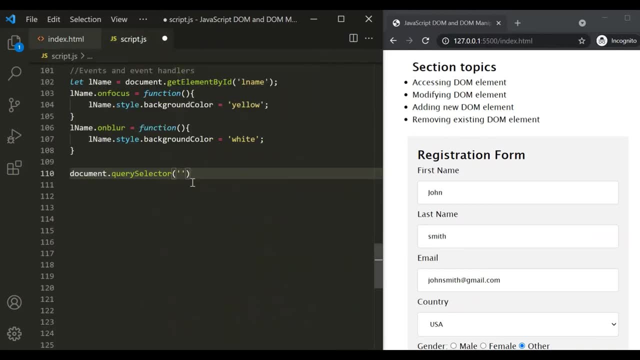 now to this. let's pass the id of this h2 element, and that h2 element is this element, so let's copy its id and let's pass it to this query selector method. and since we are passing the id to this query selector method, first we need to use pound sign and then we have. 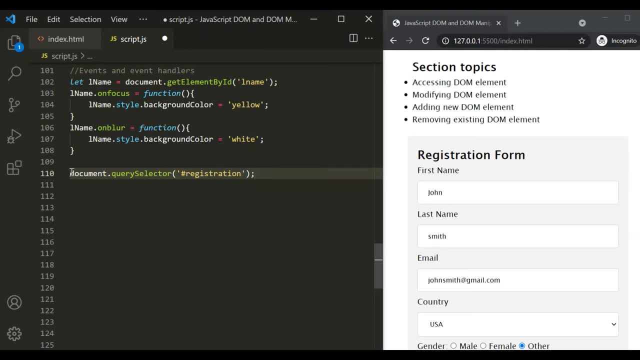 to specify the id. in this way we will get access to the h2 element- let's store it in a variable- and h2. and now on this h2 element we want to handle mouse over and mouse out event. okay, so let's say h2 dot. now the event is mouse over, so the property name should be on mouse over. so let's say on. 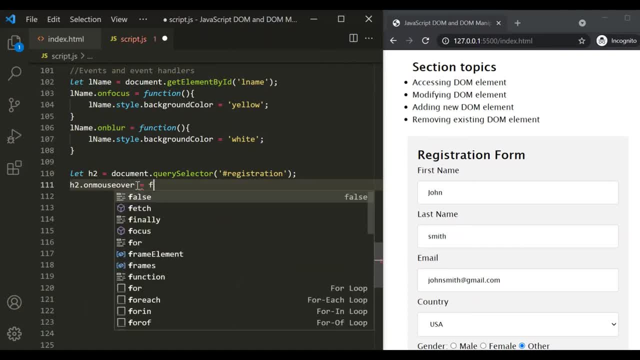 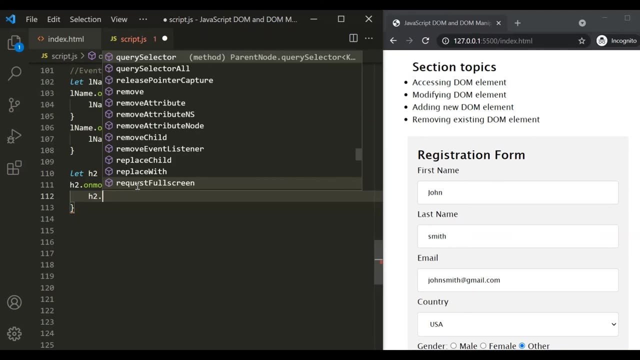 mouse over. okay, and to this let's assign a function and this function will get executed when the mouse over event happens. and inside this function we simply want to change the color of this h2 element. so let's say h2 dot style, dot color and let's set its color to. 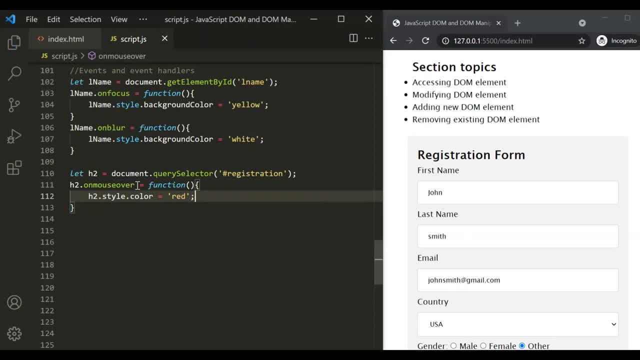 red. okay, let's save the changes. and when i hover over this you can see it's back. you know its color is changed to red, but when i move my mouse away from it, its color is not changing back to black. that's because we are not handling blur events. 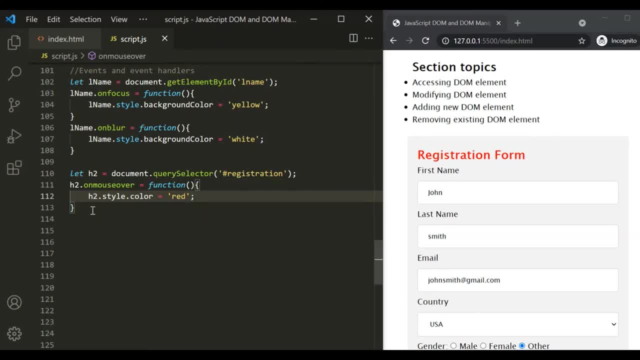 i mean a mouse out event here, so let's handle that mouse out event as well. so let's copy this same code from here, let's paste it here, and this time we want to handle mouse out event. so here the property name should be on mouse out, okay. and when this mouse out event happens, we 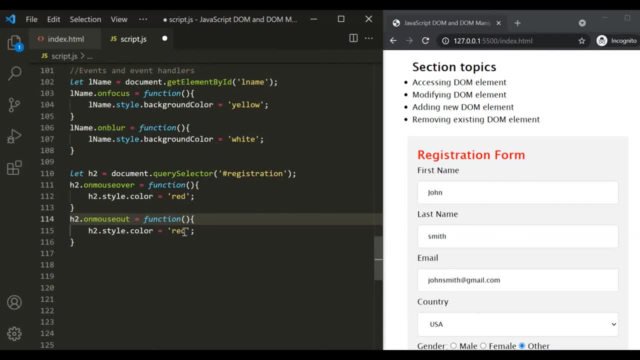 want to execute this function and inside this function, we simply want to change the color to black. okay, let's save the changes again. when the mouse over event happens, here you can see the color has changed to red. and when mouse out event happens, you can see the color is changing back to black. okay, so here we are, handling mouse.